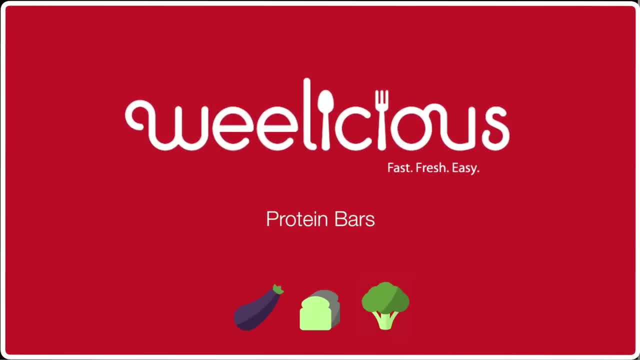 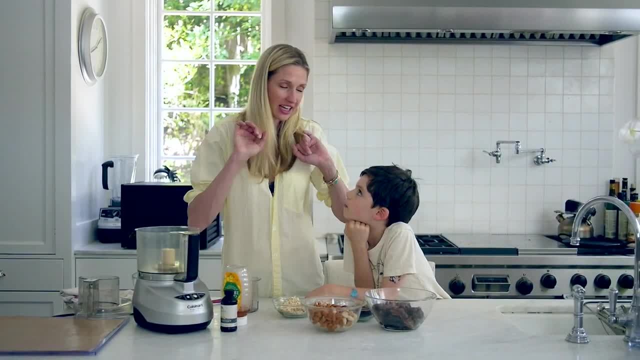 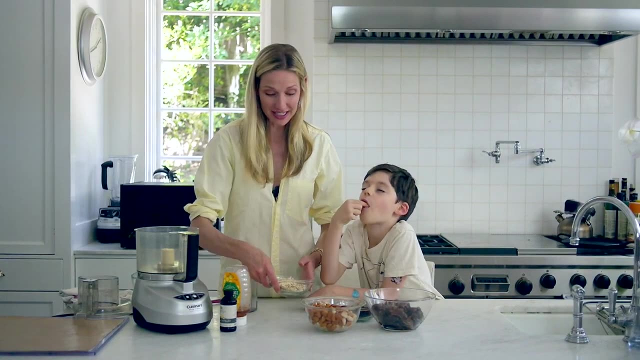 I'm going to tell you a story about when you were a little baby- and you were just a little, little little baby- I used to make protein bars and you were just in the kitchen going, nah, No face, Nothing Got nothing from it. So I started a business making protein bars. They're. 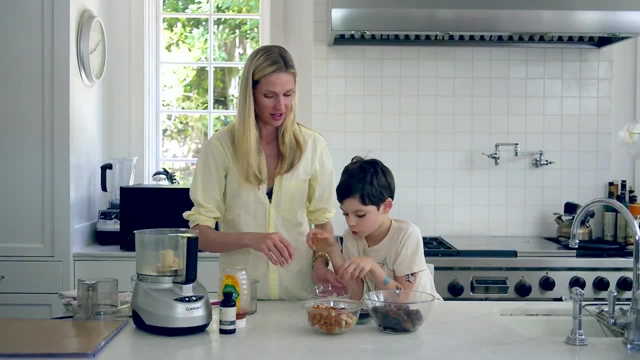 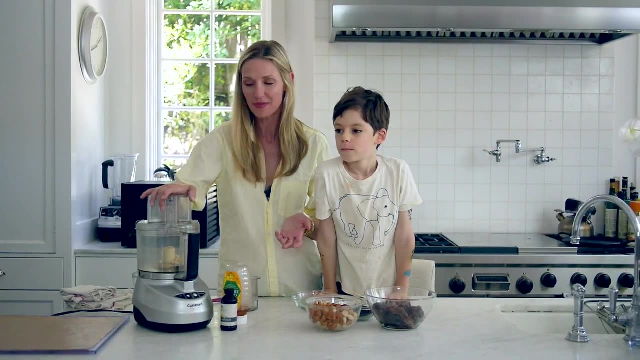 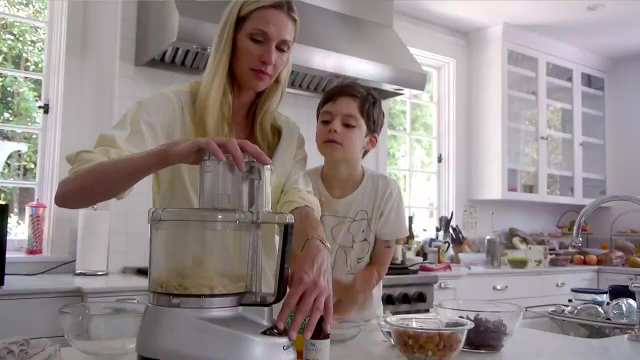 really healthy, easy. Do you need a few for you? Okay, Okay. And they're delicious and they're a great way to get protein, vegetarian protein especially. So, to start, I'm going to take whole oats, not quick cooking oats. These are whole oats and I'm going to put them. 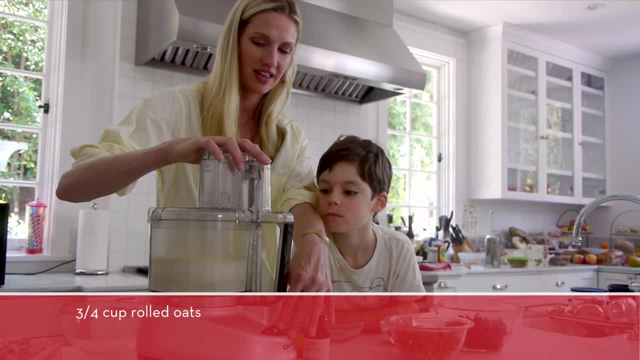 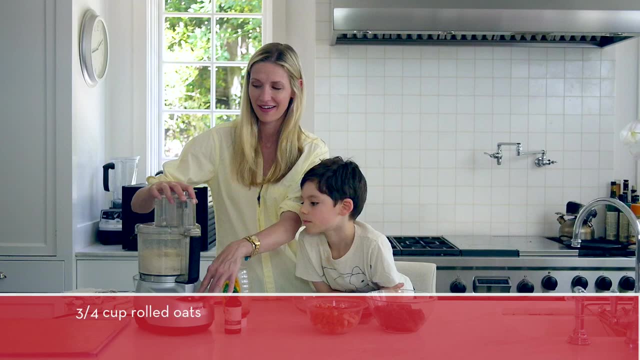 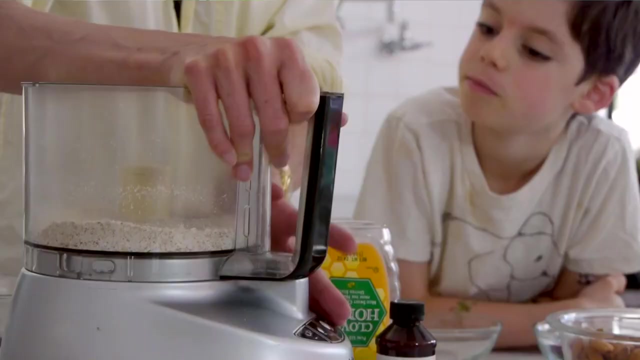 in the food processor just for 20 seconds or until they're at a fine, finely ground, And now I'm going to take them out. There's only a few ingredients, but you want to make sure they're done perfectly. Now I should take us back And can you? can I tell you? 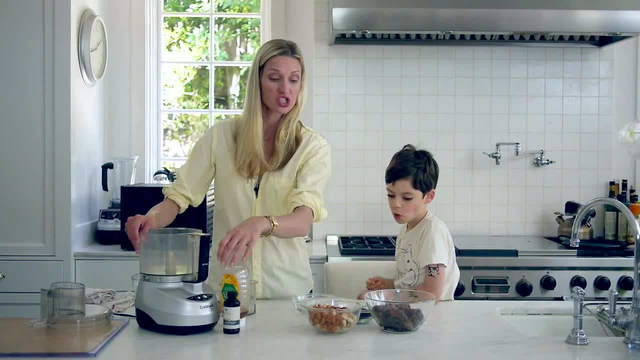 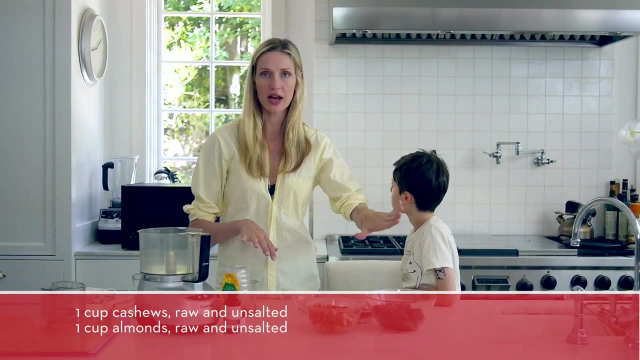 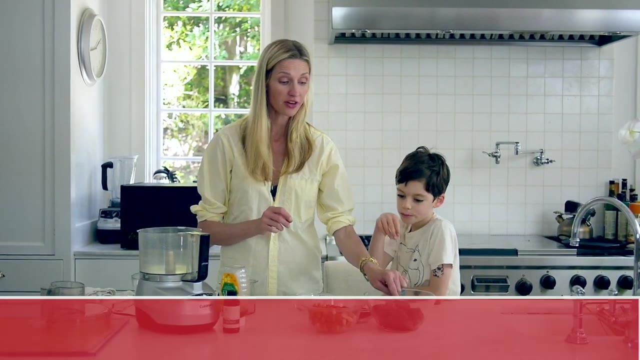 something. What I was doing earlier this morning was soaking these nuts: a cup of almonds, cup of cashews. soaked for a few hours until they're nice and soft. Drain off the water. rinse them a few times, drain off the water. 30 minutes ago I took hot water, covered these dates and then I pitted. 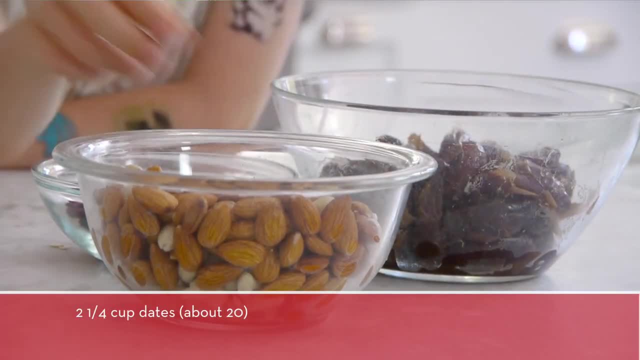 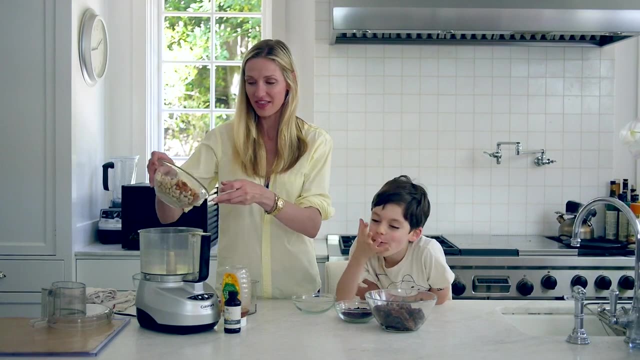 them. You want you cover them hot water because you want them to get nice and soft. How's it going over there? Okay, so now I'm going to put in the nuts, put my blade back in, I'm going to chop these nuts and these dried. 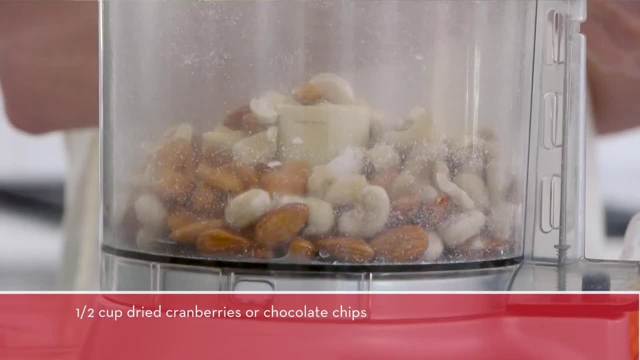 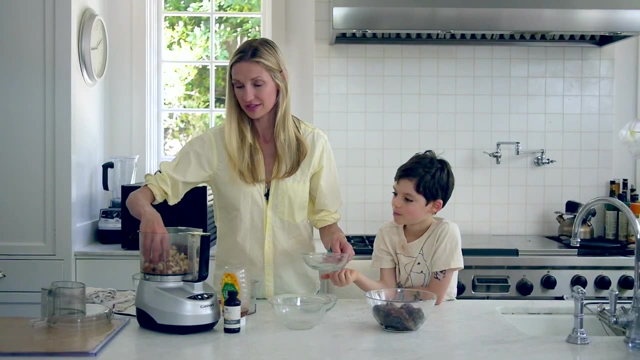 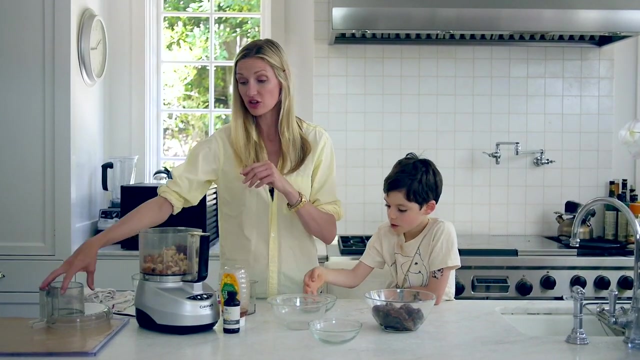 cranberries- really fine, Kenny's, never. you want some. I am going to put most of them in. You can use any kind of dried fruit. Really, Take out a few. take out a few here and there. I am going to ground them after. Okay, And then? 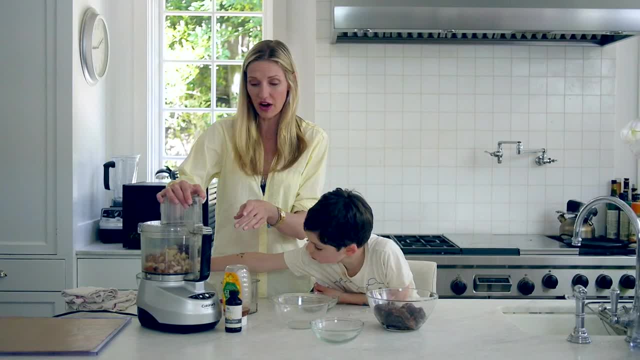 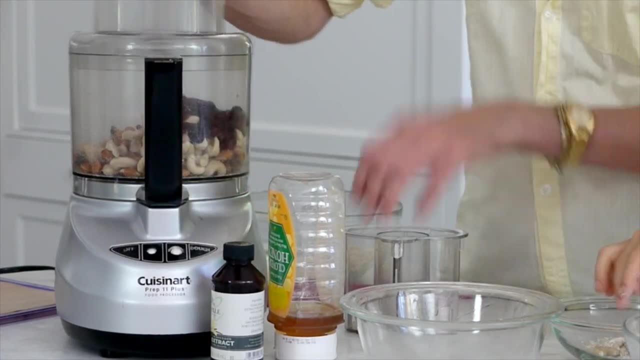 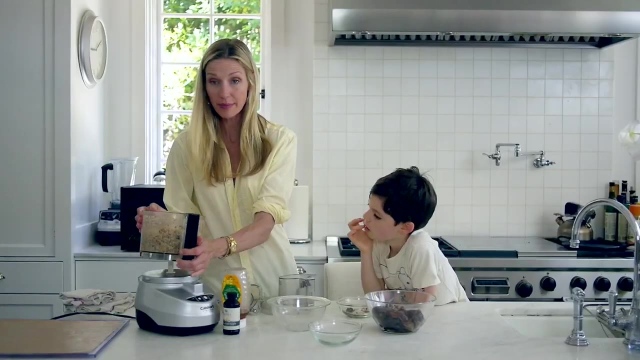 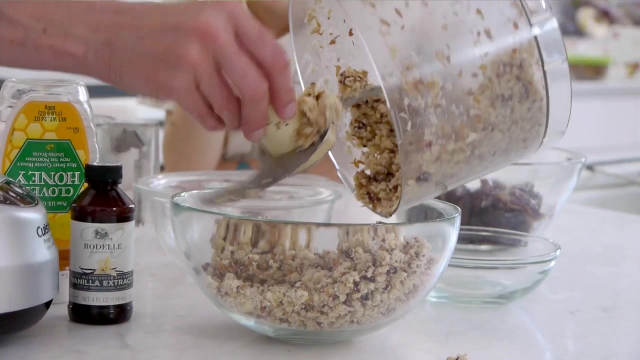 you're just going to grind this up. Okay, Fine, Not too too fine, But I'll show you, See if I can get it on. Aha, Now I'm going to take this mixture out and I'm going to add it to the oats. So, right now, now, right now, I've got the dried cranberries or the chocolate chips, whatever you want to use, Kenny is. 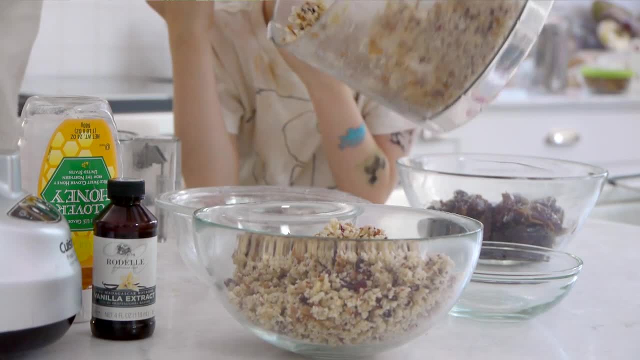 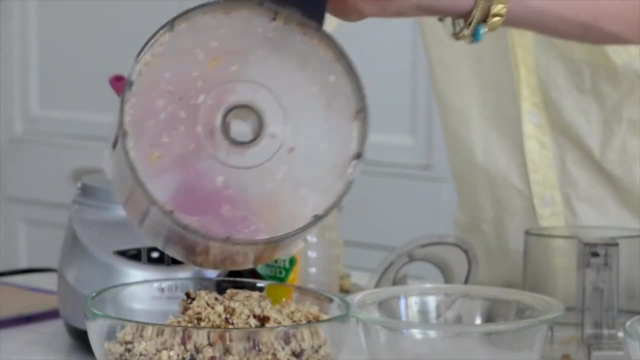 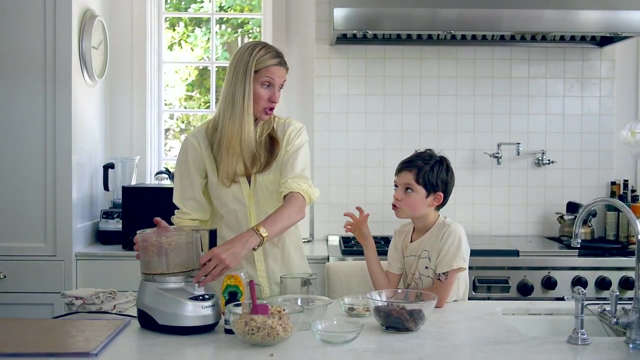 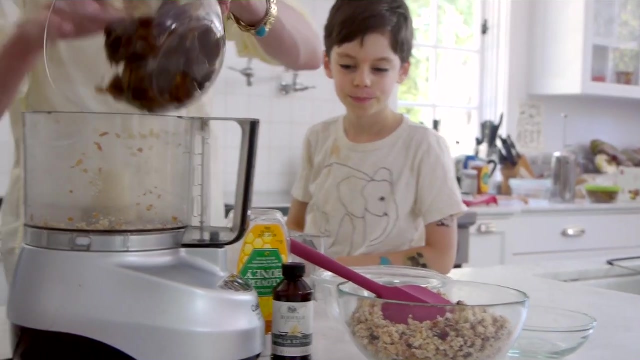 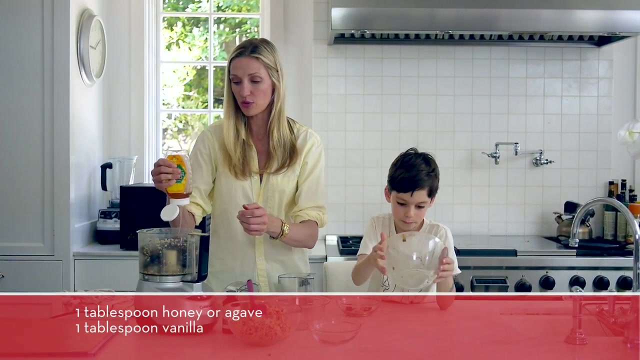 much bigger intohe likes the dried cranberries a lot better than chocolate. Not my child, Whatever Okay. And it's just because I love chocolate. I'm a chocolate girl, But I do like dried fruits too. True, True that. And now we're going to take those dates that we had soaked, put those in and we're making sort of like our soft mixture, And then we're going to take about a tablespoon of honey. That's it. If you really, if you're vegan and you don't want the honey. 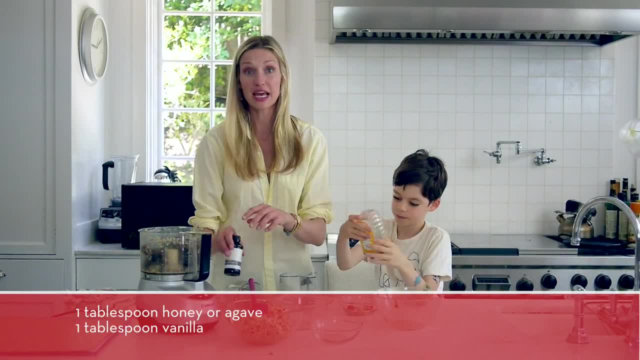 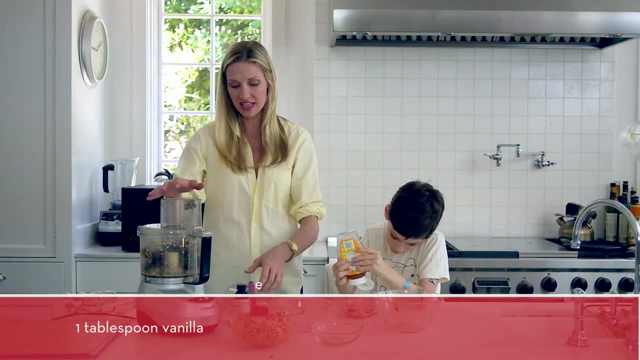 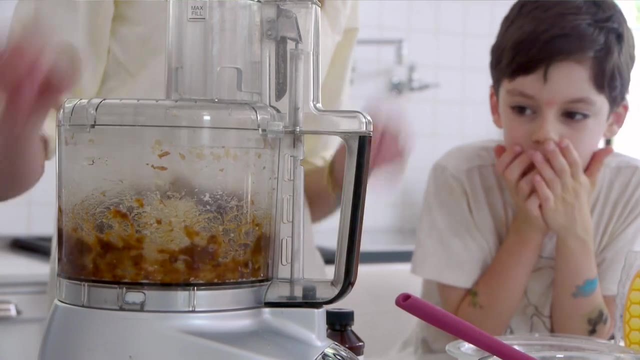 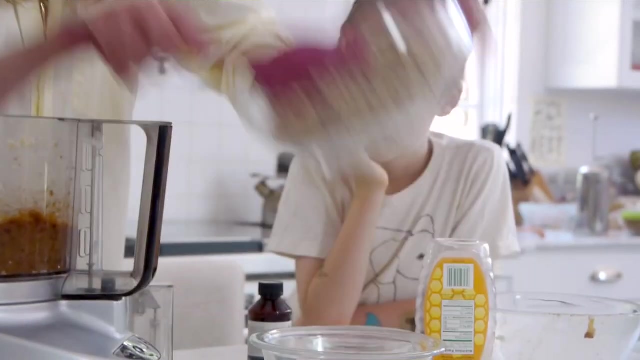 you can leave it out. Yes, And a tablespoon of vanilla extract. Okay, And now I'm going to just whiz this up until it's nice and kind of creamy. That's all you have to do. It's so nice and creamy. That only took about 20 seconds. Now you put everything in together, or you can even put it, mix it in a bowl. 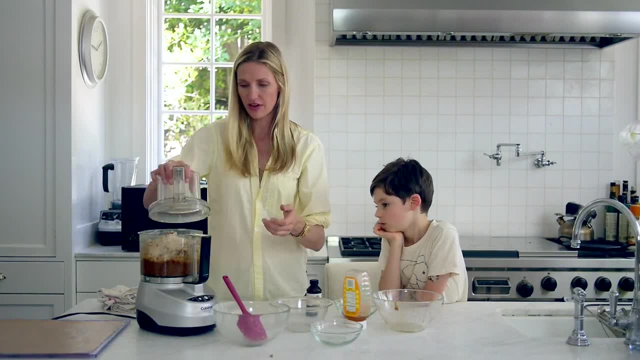 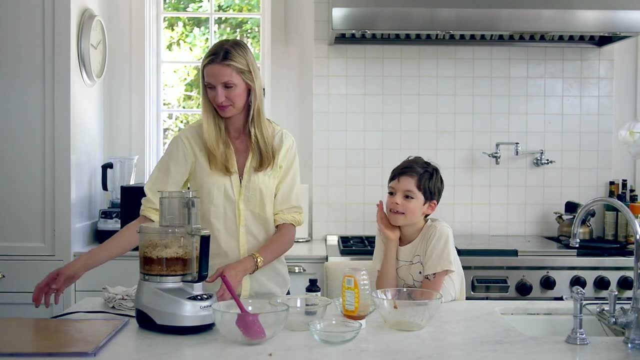 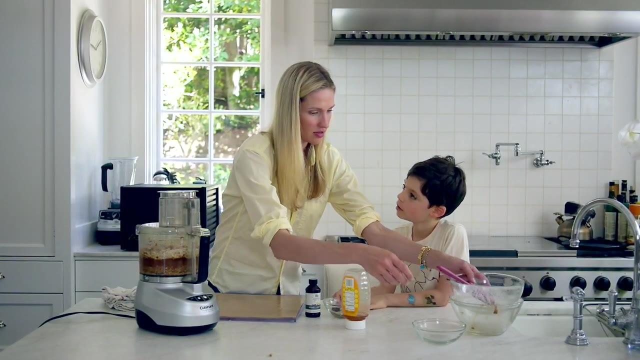 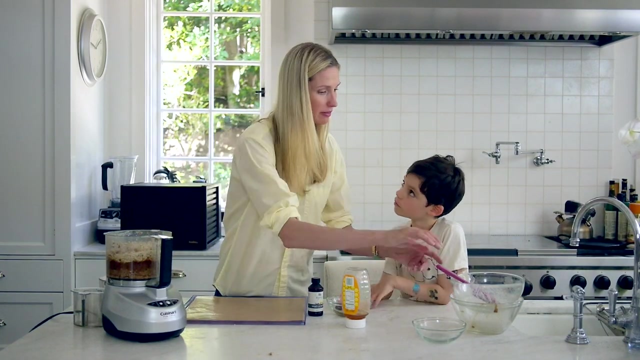 Sort of whatever's easier for you, Just give it about. you know It's going to be very loud, Louder, 30 seconds. Hey, it's not that loud. You can hear me, Mom. Yeah, After you do mine, How's that? Will you put mine in? And you know what I'm feeling like here is that that's not fully mixing. So what I'm going to do, You want me to mix mine, You want me to mix yours. 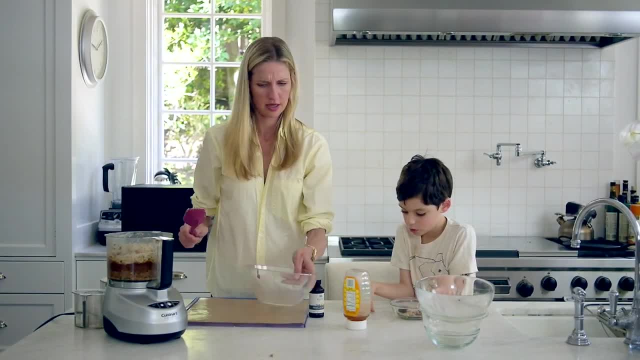 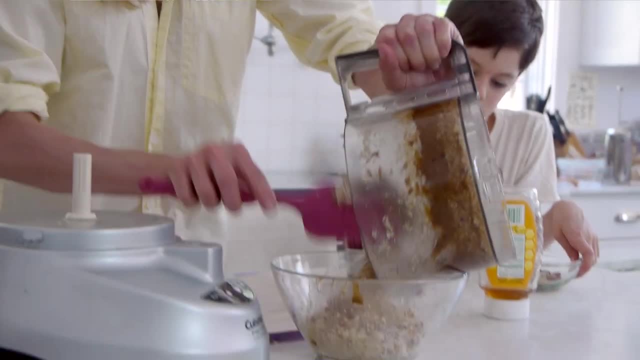 I'll put mine in. I'll put it in. Why do you want me to put yours in? Well, why don't you eat it like that? I like how you made that sort of deconstructed mixture, And what I'm going to do is take a few seconds and stir this all up till everything is totally combined. 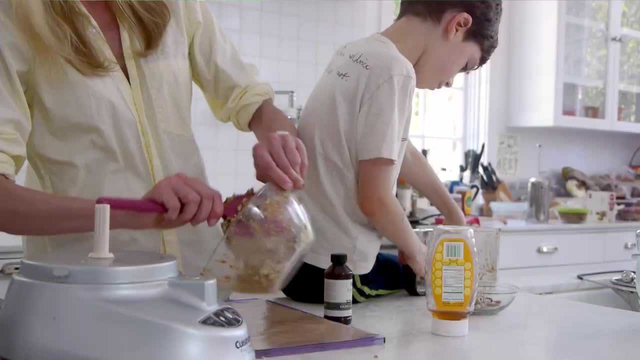 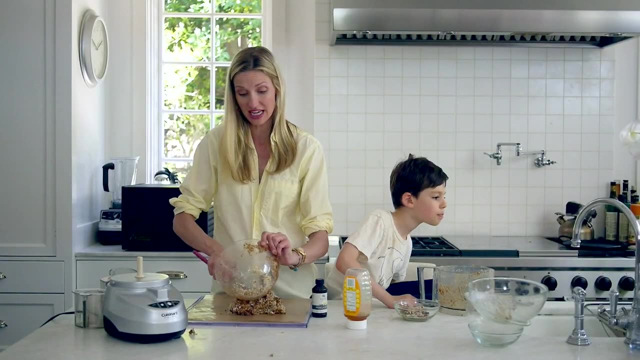 All right. So now I've mixed up the mixture, I'm just going to place it on this Silpat. you could use. this is a special sheet that goes with the dehydrator, and but you could also put it on a silpat and bake it at 200 degrees for about four. 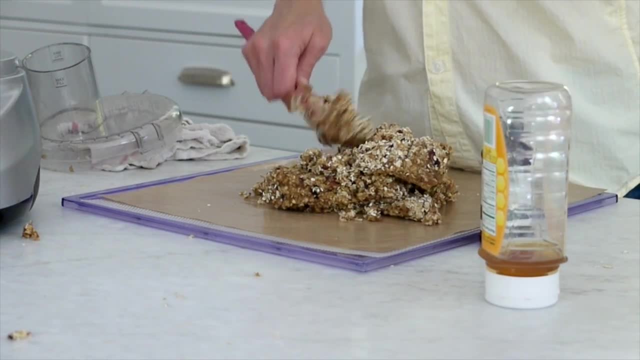 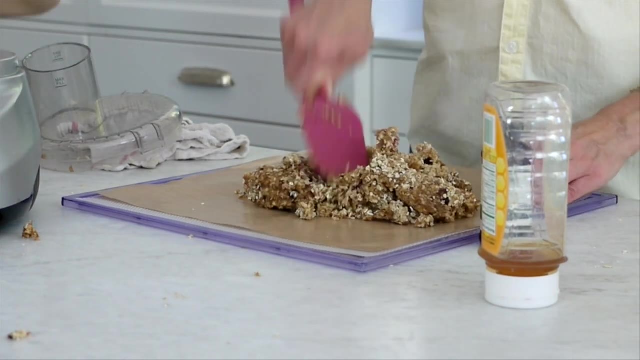 hours, because what we're trying to do with this is bake it, but not so much that it's truly baked. it's not going to become hard, it's just like a protein bar, nice and soft. what, when? you're okay, hold on one second, cuz I'm gonna take these.